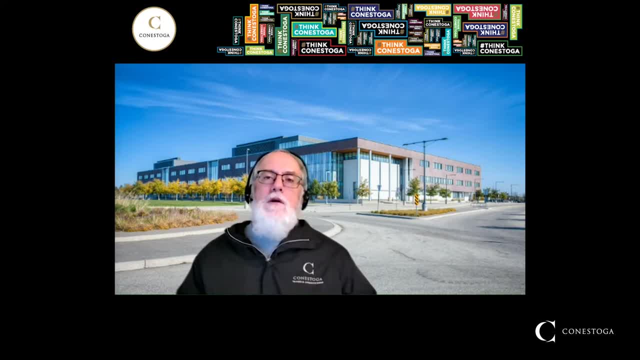 and fabrication world. The Welding Techniques program is a one-year program that introduces you to that field. If you'll bear with me for a short presentation, I'll explain more about the program and I'll also provide some contact information, and you can also 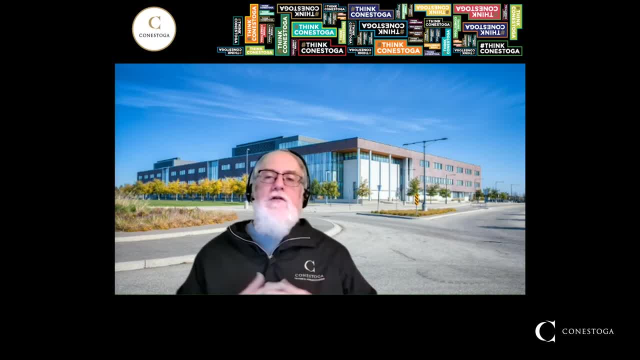 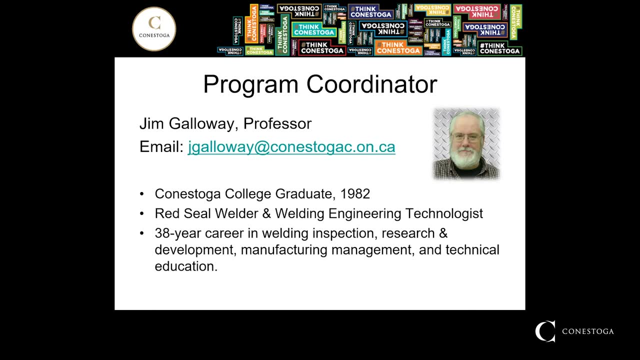 find your way to virtual tours of our facilities so you can see what's inside those four walls. Thank you for your time today. At this time I'd like to do a little introduction to myself as program coordinator. but I want to emphasize: I'm only one person on a teaching team. 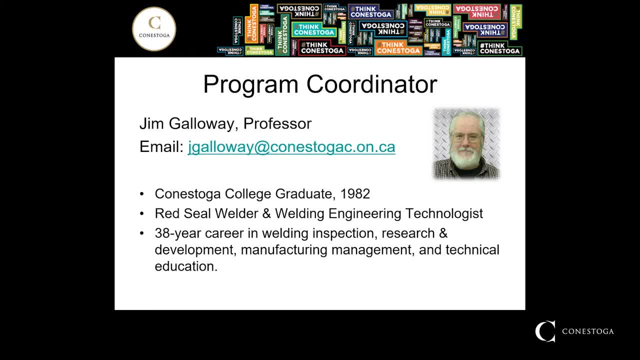 We have experts in metal fabrication, engineering drawings, welding skills, welding process theory. All the different experts work together as a team to teach students. For myself, I'm a graduate from Conestoga College, Hanasoka College. I graduated from the welding tech program back in 1982.. After that I earned 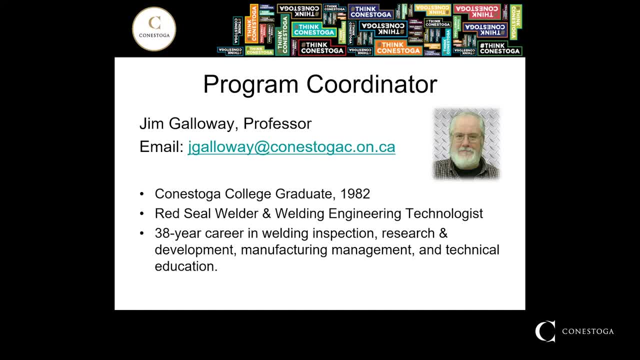 a welding red seal, but I'm also a welding engineering technologist. I've also earned some other credentials in welding inspection and whatnot, but that's the primary credentials that I have. I've worked in this business for 38 years. I started off as welding inspection at a nuclear 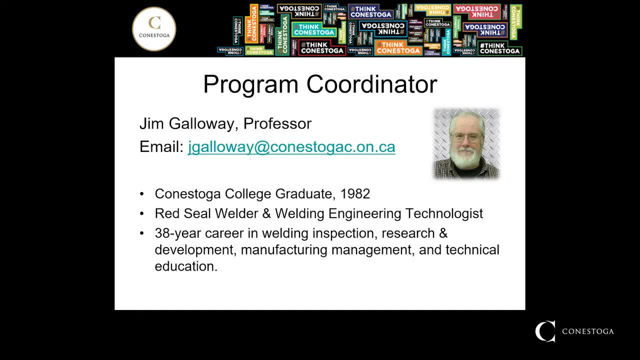 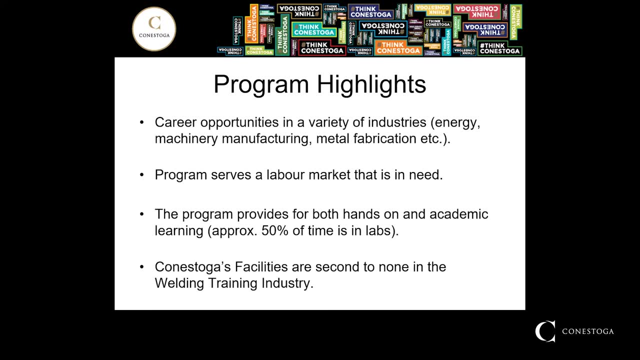 power plant construction project, but I've also worked in welding research and development and I've been a manufacturing manager in a couple of plants. Most recently, obviously, I've been doing technical education. In the next few slides I'd like to give you some highlights to the program. 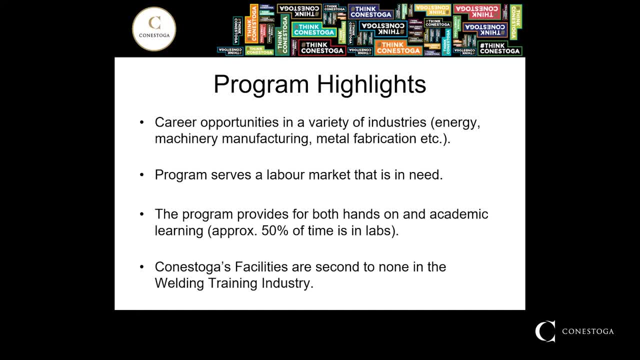 We're going to look at pathways that students have when they complete the program or in the education world. there are also career paths. But the bottom line is students are looking for good careers and in the welding industry there are good careers. locally. There's still a high demand for welding and fabrication skill sets. 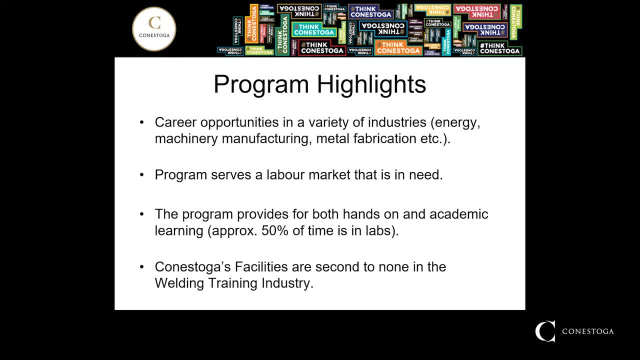 so we've set up our programs to fulfill that need. We work very closely with industry on our program advisor committee and equipment suppliers to give the students the knowledge they need to be successful. The program is over 50% of the time in the shop doing hands-on work. 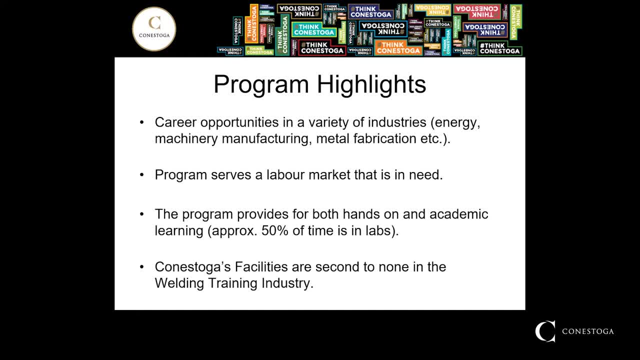 practical work Supported by theory, which is important to understand: safety processes, engineering drawings and all those support courses. You'll see we have the virtual tour, that we've got an excellent facility. We've got lots of welding equipment, big shops. every student gets their own welding booth that's well ventilated. 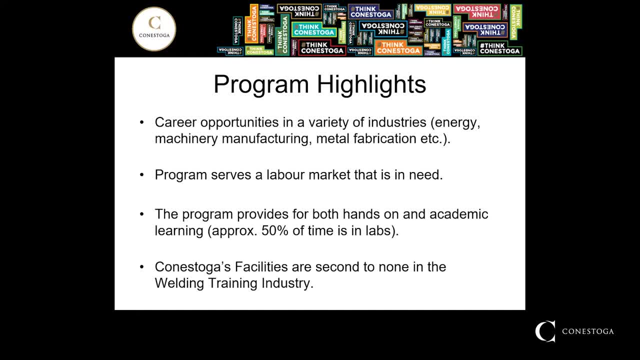 We've got a welding technology lab, we have a big metal fabrication shop, we have a welding robotics facility and also a welding and inspection lab. All of these are facilities that we've built up and that makes our program one of the strongest in the country, certainly in Ontario. 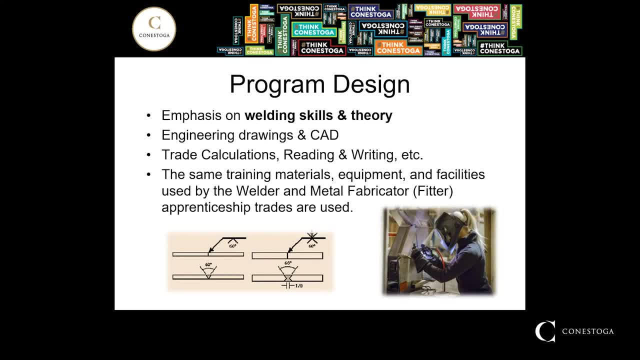 Conestoga College's Welding Techniques program is a one-year program. It starts in September and students graduate in the spring. The focus of the program is on welding skills development, but also with any trade. we also include a theory component. 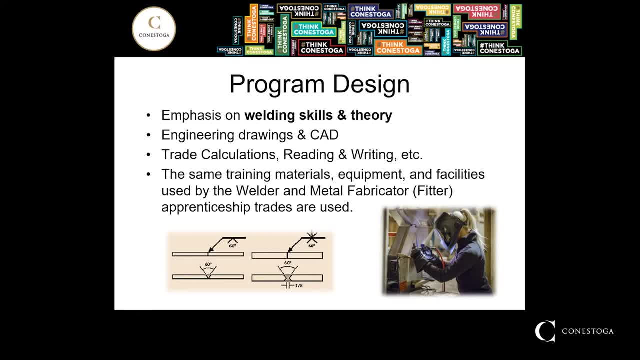 It's important for students to understand safety, Welding process, settings, gases, electrodes- all the important considerations that must be to meet an employer's expectations. Most employers expect welders to read prints, so we teach engineering drawings. All Ontario College programs include trade calculations and reading and writing skills development. 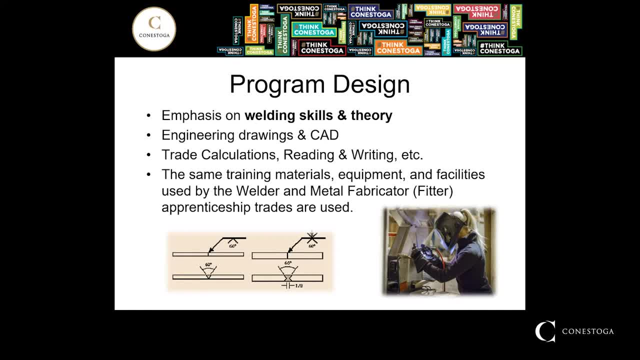 So that's the emphasis of our program is building welders, teaching them the theory And getting them into the trade. However, our unique approach is to also use the same training materials, facilities and equipment that we use to train welder apprentices. 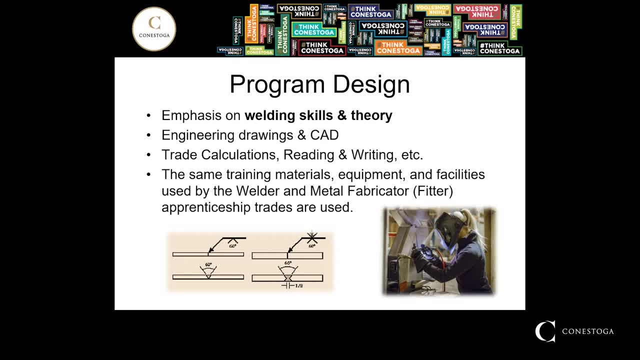 So Welder and Metal Fabricator Apprenticeships, trades, are also available at Conestoga And I'll explain more about that process later. But the Welding Technices program is really your first step into this business, So we try to as much as possible accommodate the students needs. 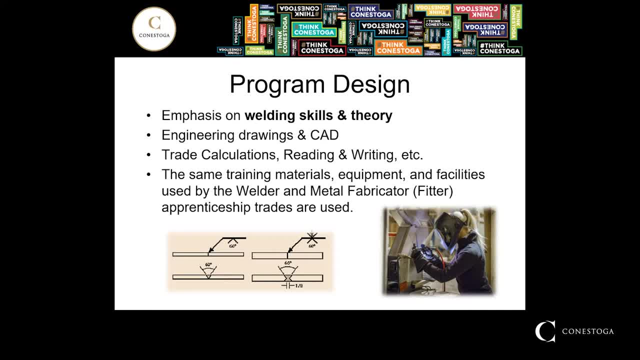 And build their skills and theory knowledge up so that they can apply the trade also. you'll learn more as we go through the presentation. there are opportunities to take the credits earned in the welding techniques program and apply them to other programs for advanced standing. you'll see as we go through this. 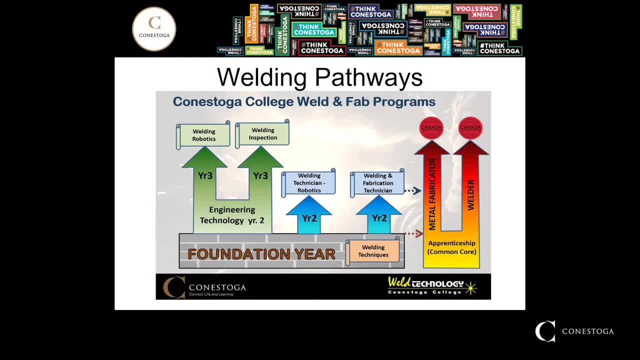 presentation. one of the key advantages of the way the welding programs are structured at conestoga college is the integration of the programs. it's called laddered learning. students have the option of starting into a welding techniques program, which is a one-year program, so you'd earn an. 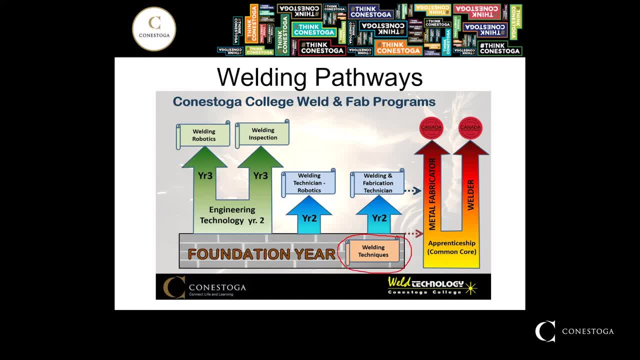 ontario college certificate. after one year in welding techniques, those students have the option of continuing on in other programs. provided that their marks are equivalent to the first year of the technology- math, which requires a 70 percent, they could go into these two programs. these are three-year engineering technology programs, one's targeted at welding robotics. 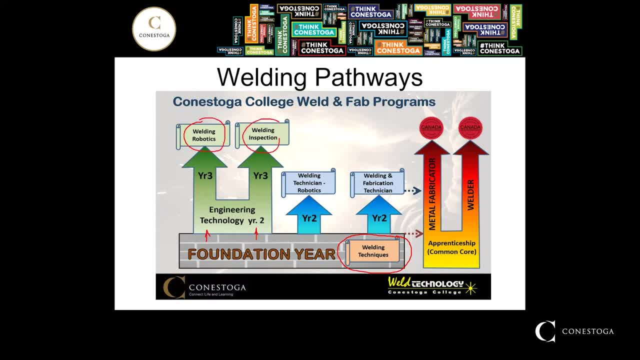 and the other ones target at welding inspection. but these are engineering technology programs, and so the requirement would be to achieve at least 70 percent in the first year. math courses called trades calculations, but that's certainly possible. we have students that do it all the time. another option is to take the two-year welding and robotics technician. 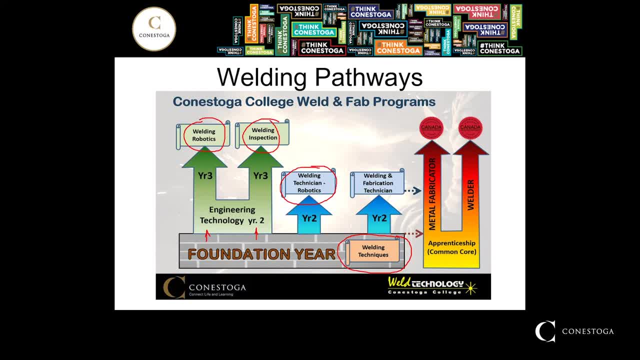 this program has less emphasis on engineering, but it does have a strong emphasis on welding automation. this is a new program and you would not have to achieve 70 in math. just pass those courses with a minimum of 55 percent, so these students could then transfer into that program, or they. 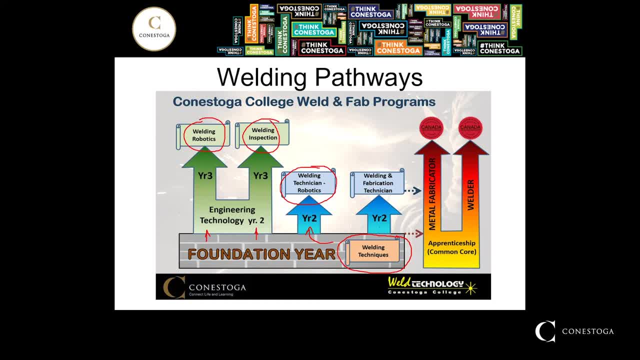 could continue on in the welding and fabrication technician. that's a two-year course with an emphasis on metal fabrication in that program in the second year. So this foundation year then establishes the baseline skills for all the students in all the programs. They're all in the same welding skills courses and they're in the 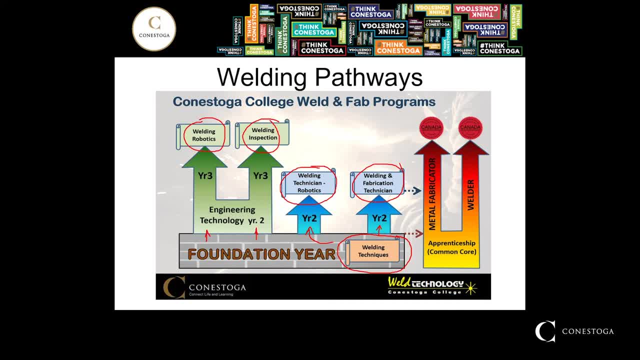 same welding theory courses. The only difference is the engineering technology students take a different math course. So there is a pathway then for students in any of these programs after the completion of year one to continue on in another program. For example, a student in welding and 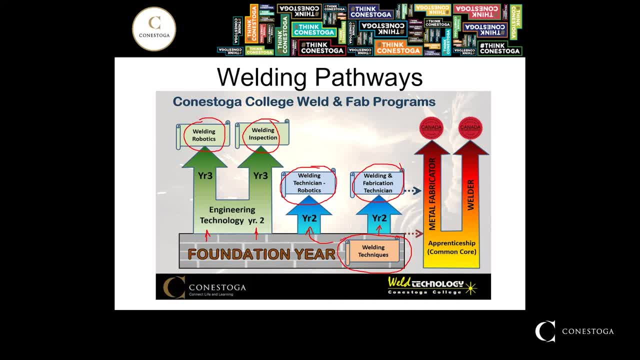 fabrication technician that decides to switch can go into this program, and if they achieve over 70% in math, they can get into either one of these two programs. So these are all options. Another great option is that if a student who is in the two-year program one of these programs decides 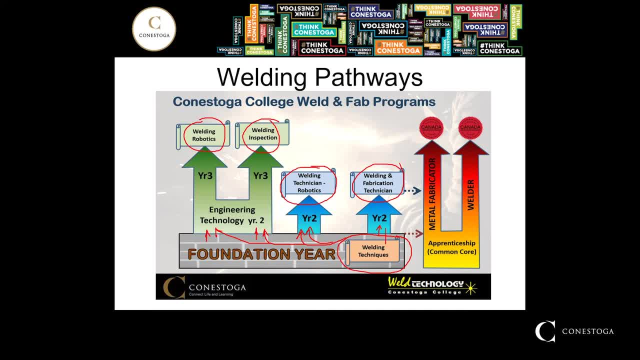 not to continue on. they can then graduate with welding technique certificate and complete their college program with a certificate. Another important option is the ability for students to go into an apprenticeship. So the pathway is here. These are exemption exams. We've structured our programs to be compatible with the Ontario 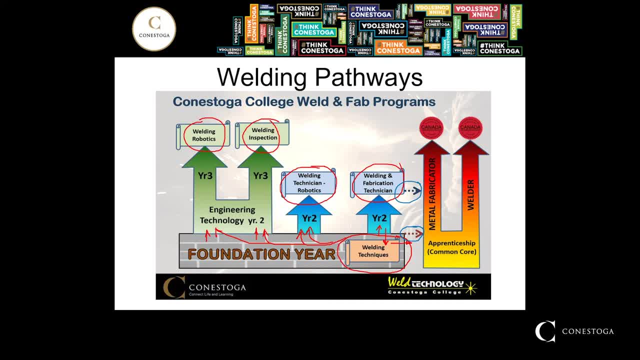 apprenticeship curriculum for both the metal fabricator trade and the welder trade. As you can see, these two trades have a common basis. For example, we have a metal fabricator trade and a welding trade. As you can see, these two trades have a common basis. 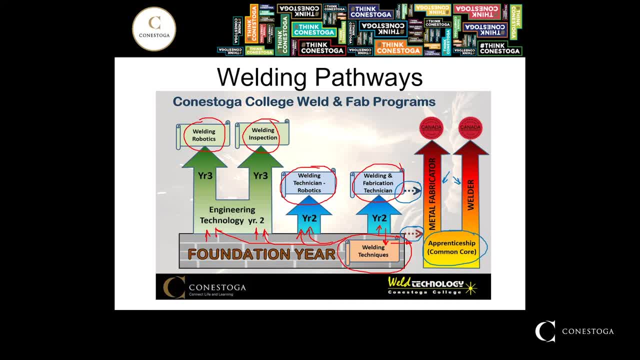 These two trades have a common basis. For example, we have a metal fabricator trade and a welding trade. As you can see, these two trades have a common basis. These two trades have a common basis. The nya three are basically fixed at the same time. The new level beta gamer can't apply to exception. 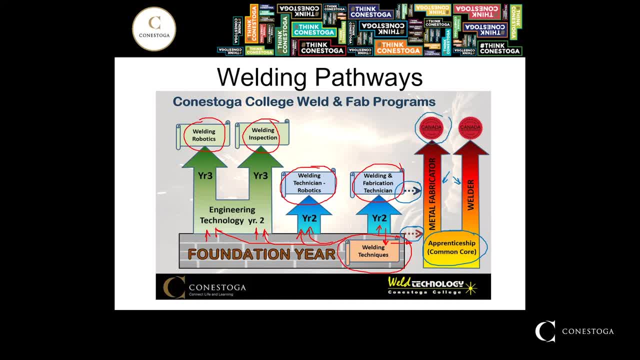 programs such as welding and fabrication. so departing a company has a common basis in working people from Empire to America. five things to keep in mind when applying for the programme of FlexGraph, Canada's butcher construction. So the students then, at the completion of the program, could apply to red exemption exams that would give them advance standing in the apprenticeship. after working as an apprentice after a company, earning experience, they could also 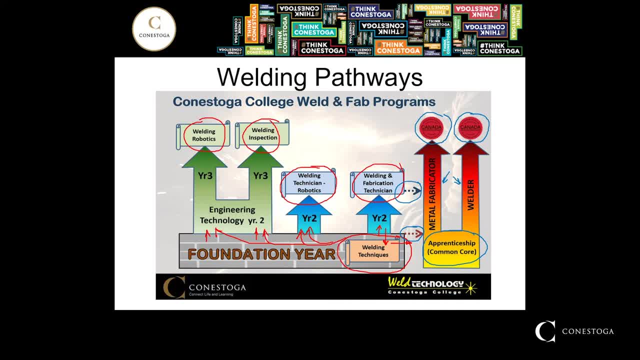 So the students then, at the completion of the programme, could apply to retrouver funds up to twenty insurance in the program to help out against a grupo where there's several consists. after делas ay ay ay. after the completion of a three-year apprenticeship with the work experience, 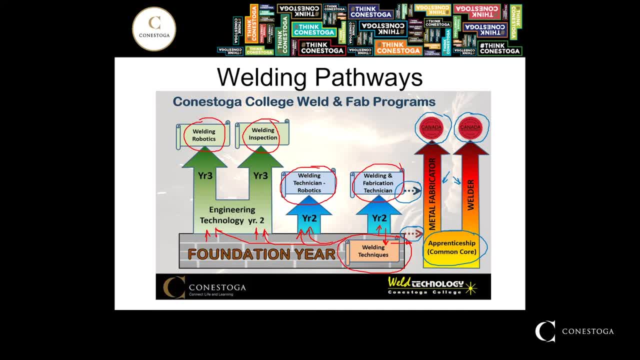 those are all options, so the pathways have been established. we call it laddered learning or stackable credentials, and it gives the students a lot of flexibility. we have many students who enter the first year of the programs not really sure what they want to do in their career and once they learn more, 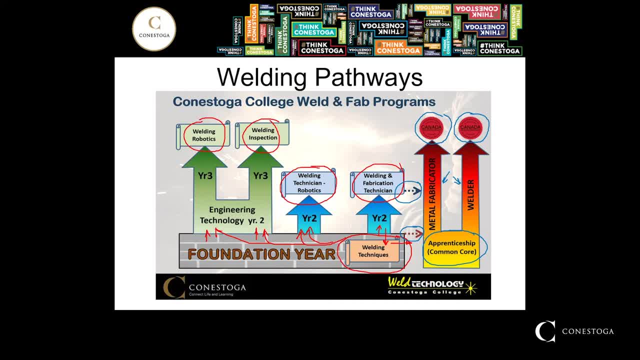 about something like welding robotics or welding inspection. we see a lot of students that request to switch over and will allow it, provided they have all the credits and provided there's room in those programs. we've never turned anyone away yet, so this is a strong advantage of the Conestoga College welding. 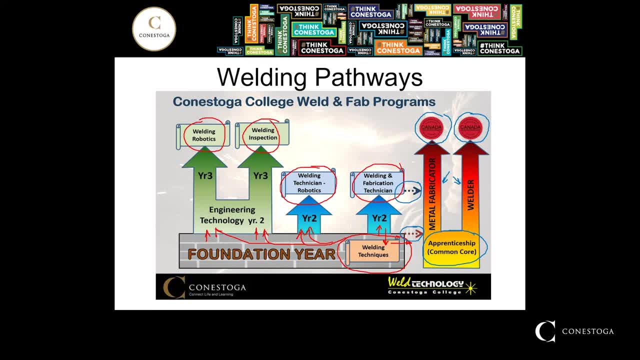 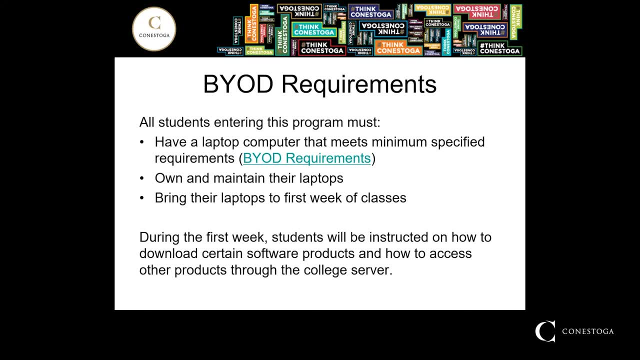 technology programs. one of the new requirements in most programs in Ontario is a need for the students to bring their own device. this basically is a laptop. many students already have laptops, but it depends on the program requirements programs. various programs are required to bring their own devices to the school. so we 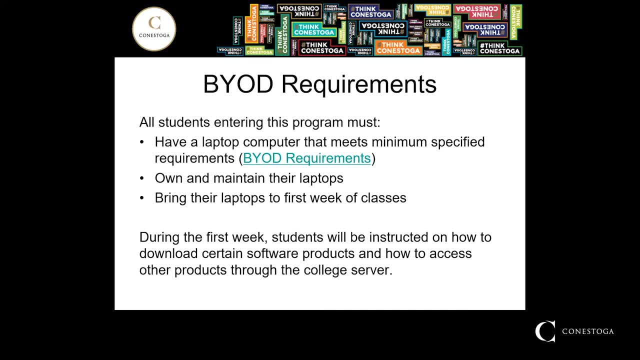 vary from program to program in terms of the software used. in our program, we're recommending a machine that could run the most advanced software that we require. most of the applications are Microsoft and fairly general. however, as you'll see in the next slide, we are requiring that the students have a 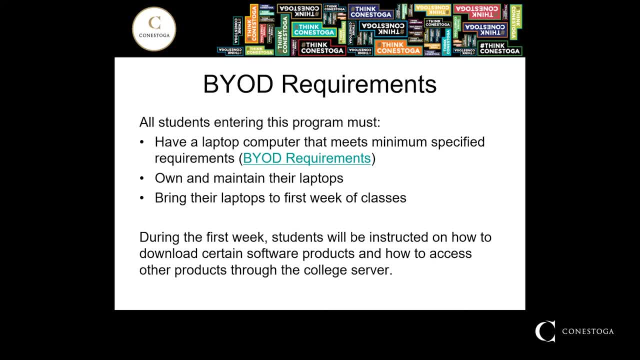 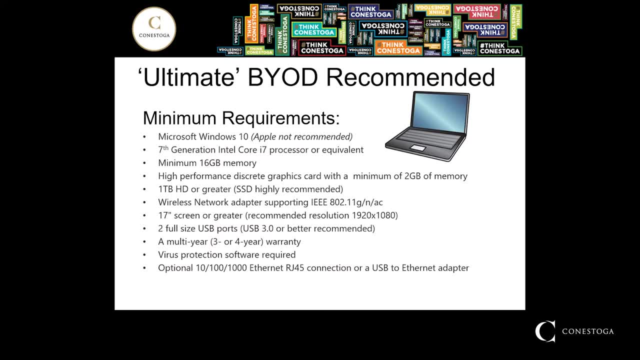 machine that can run AutoCAD and SolidWorks. on this slide you can see the specifications for the laptops that we're recommending for students to bring with them for school. in our case we run certain software- AutoCAD, and and also SolidWorks- and these are fairly computer intensive, so we're recommending this. 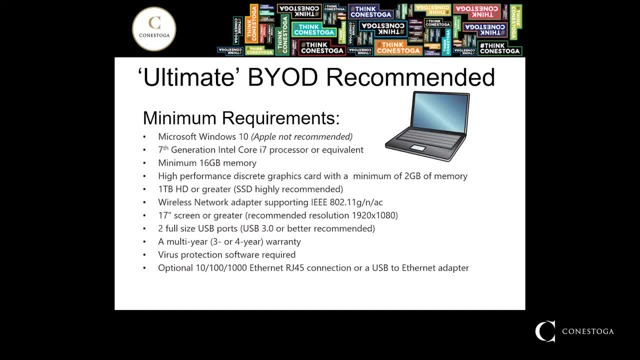 minimum requirement. one thing you'll note that may vary a little bit from what you see on the website is that we're not recommending Apple products based upon some conflicts that we've seen with students trying to operate the software using an Apple product. apparently it is possible, but it's just one of these. 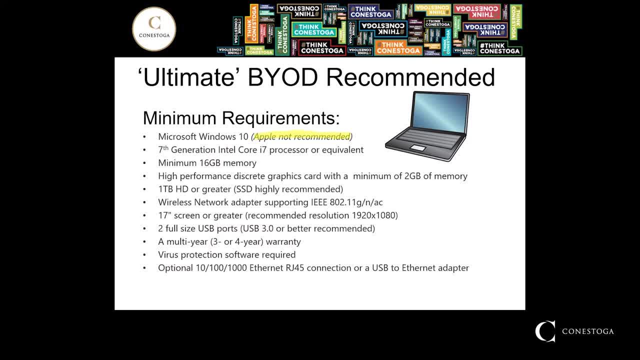 hiccups we're trying to avoid. I'm not a computer geek, but for those that are knowledgeable at computer, you can basically take this information to any computer shop and they will be able to help you acquire the proper technology. there's more information on the college website as well. over the next few slides I'll be giving you this. 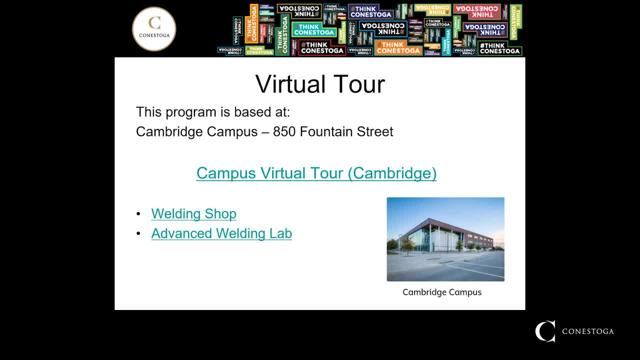 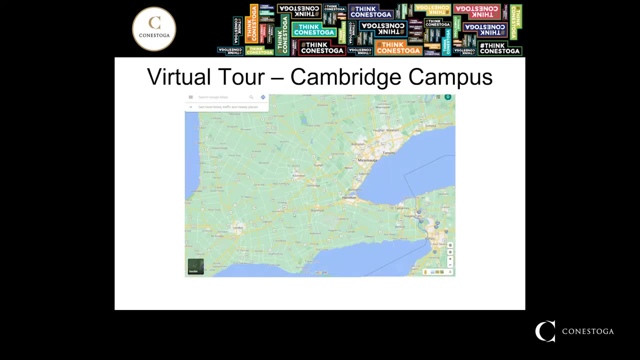 virtual tour of Conestoga College's Cambridge campus and our welding facilities. I encourage you, though, to click the links yourself. they're available through the link below to the program page on the college website. you can then explore the campus yourself and look at the other facilities. so first I'd like to locate. 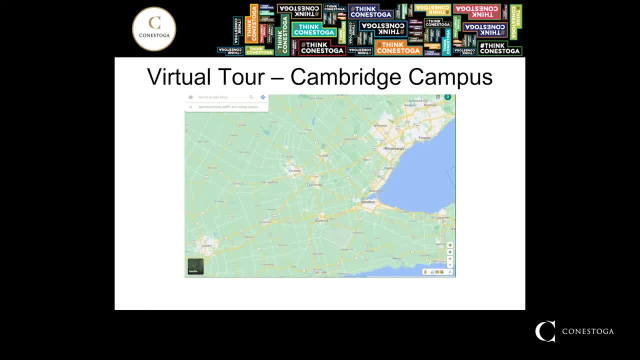 where we are. we're at Conestoga College's Cambridge campus. so let's zoom in on Cambridge. you can see we're near the south end of Kitchener and the north end of Cambridge. we're right off the 401. let's zoom in on Conestoga. that's our. 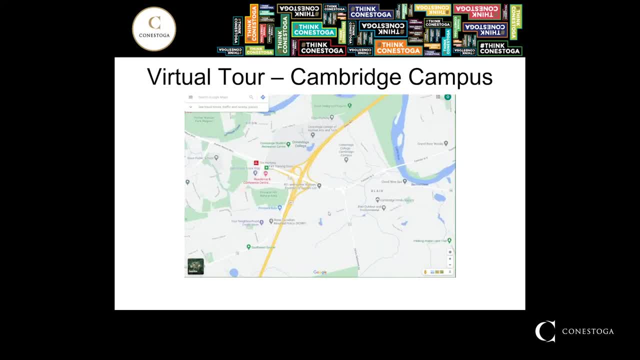 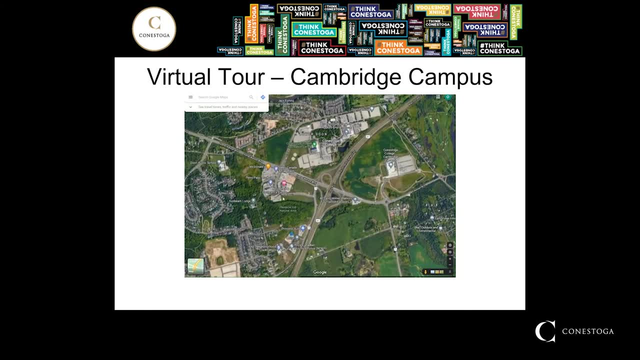 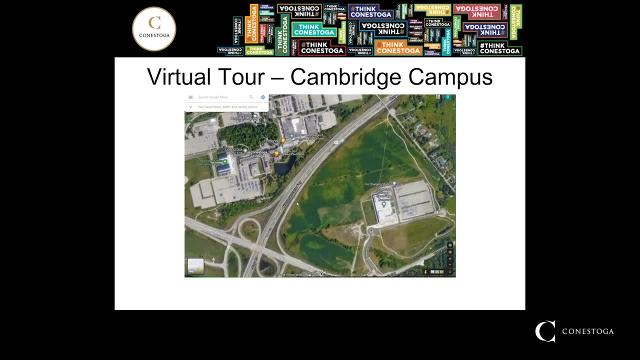 Dune campus and we're basically in that location near Homer Watson and the 401. let's have a look at Google Earth. there you can see the college residence. that big area is the Dune campus. we're on the other side of the highway. there is a 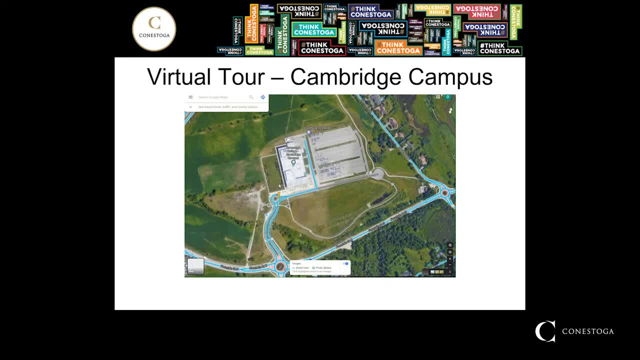 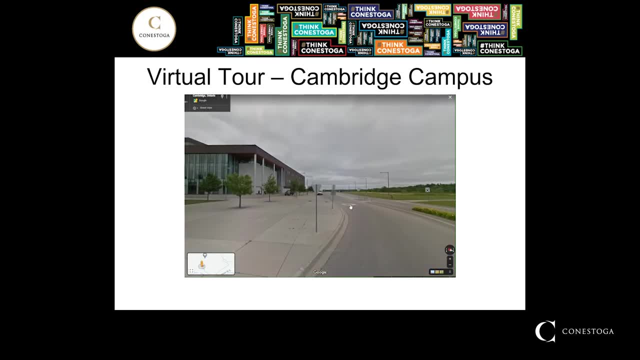 shuttle bus between the different campuses. let's zoom in on our campus. here were near the roundabout at the campus, near the roundabout at the corner- that's the front of the building. there's a bus stop right in that area. let's go around the back down in this area. you can see. 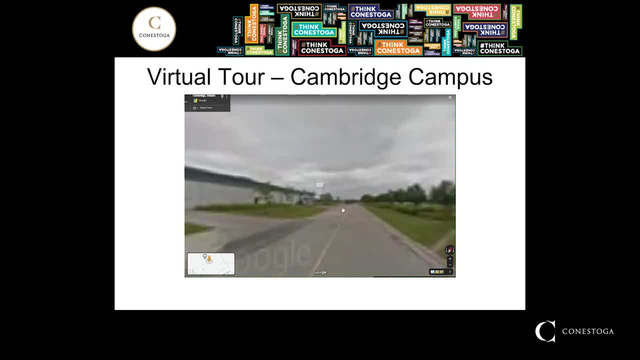 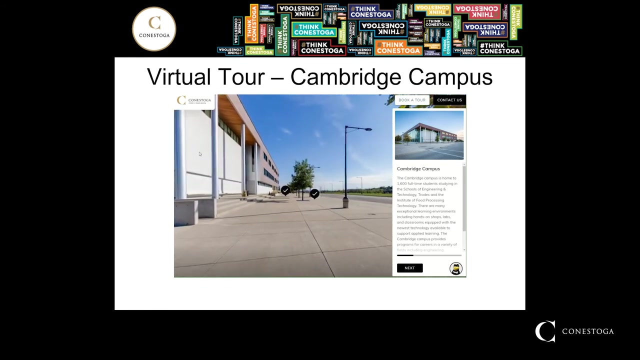 the entrance from the parking lot and that white wall is the shop areas. here you can see the welding shops, those big ventilation systems. they're basically there, our exhaust system to keep the air clean in the shop. this is the start of the virtual tour of the Cambridge campus. here we're looking alongside the 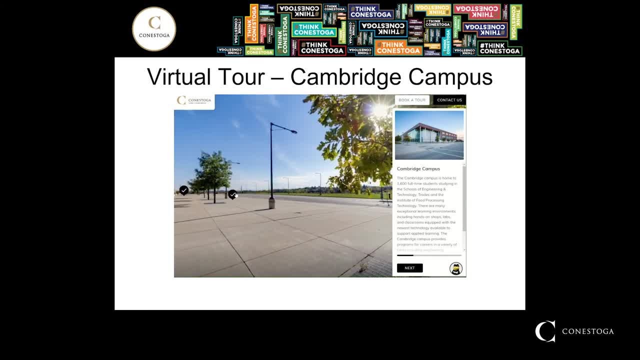 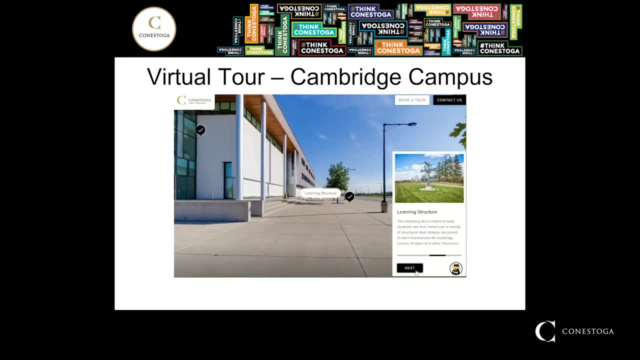 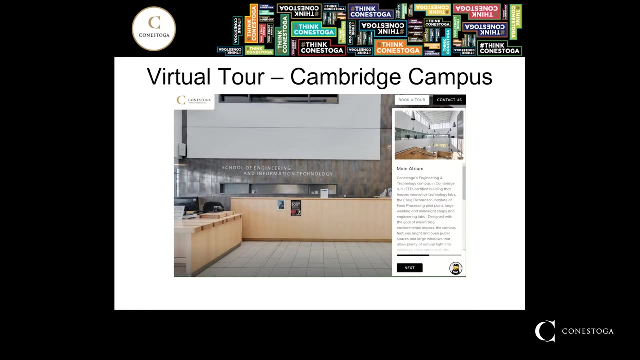 building. we'll go back and have a look. this is the front entrance to the building. we encourage you to have a look yourself again. the links to the virtual tours are available through the college website or the welding program pages. let's have a quick look around the main floor. this is the lobby, the atrium, that's. 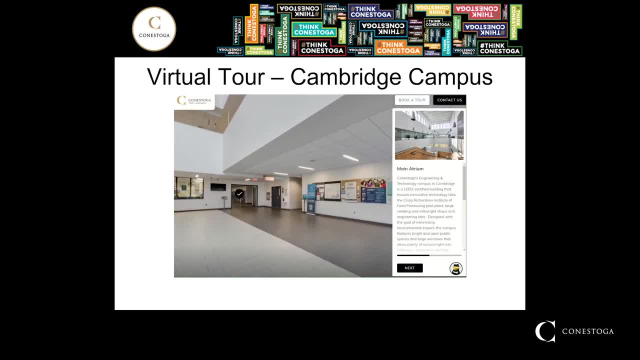 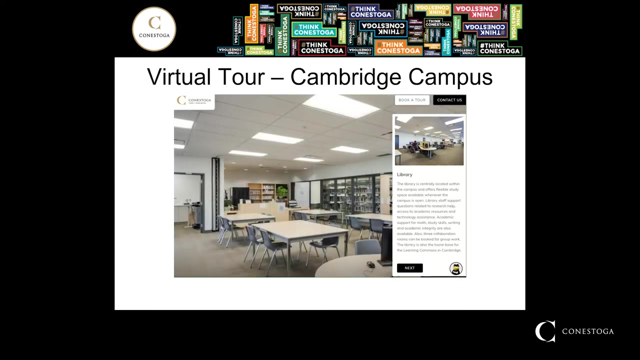 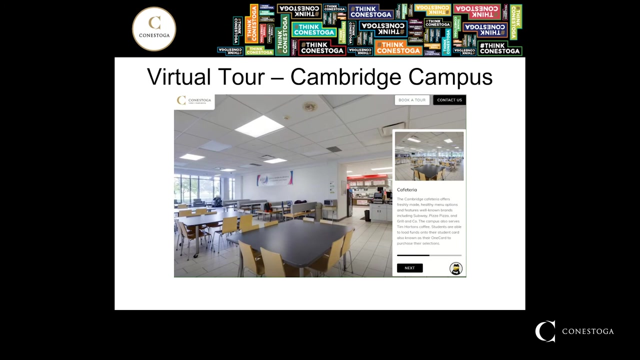 Conestoga Students Incorporated's office. this atrium is three stories tall. there are actually three floors of classrooms. all the shops are on the main floor. let's have a look at some of the key service areas on the main floor. that's the library, here's the cafeteria. 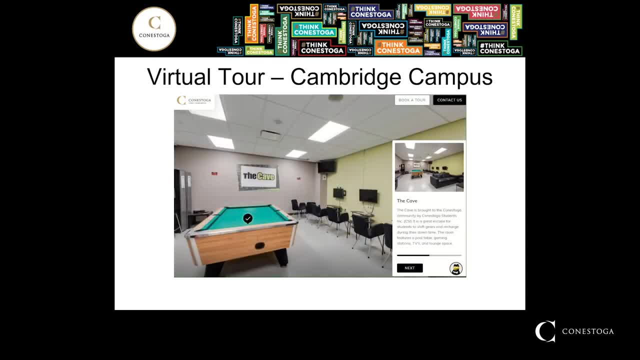 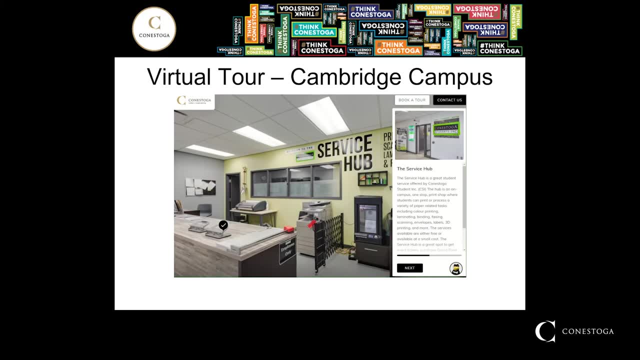 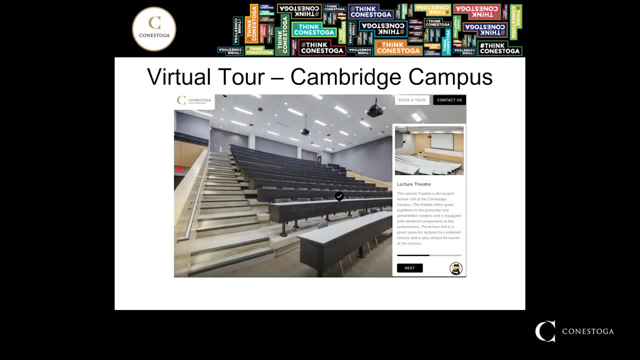 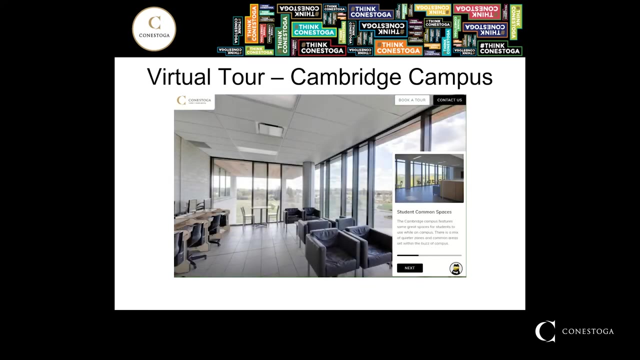 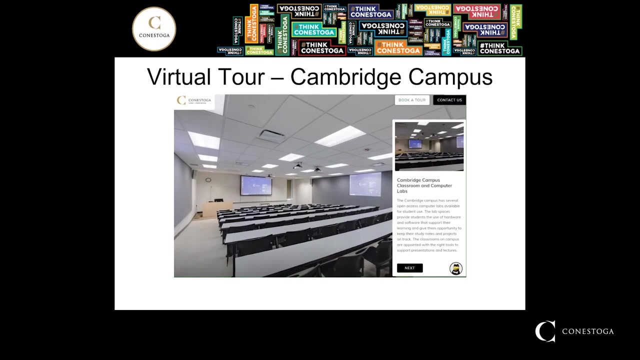 you, you. This is the student lounge. This is the service hub sponsored by Conestoga Students Incorporated. This is an example of one of the large lecture theatres. Here is a study area for students on the second floor. This is another large lecture theatre. but I will tell you, in our programs we typically 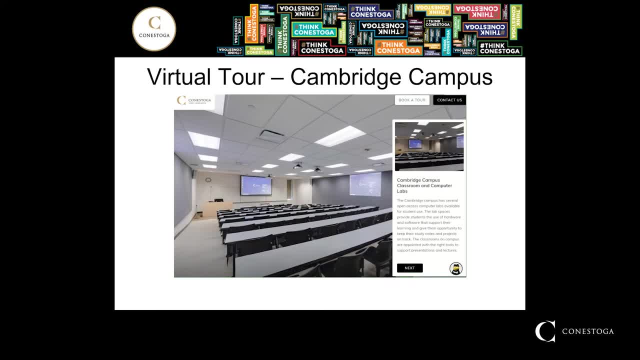 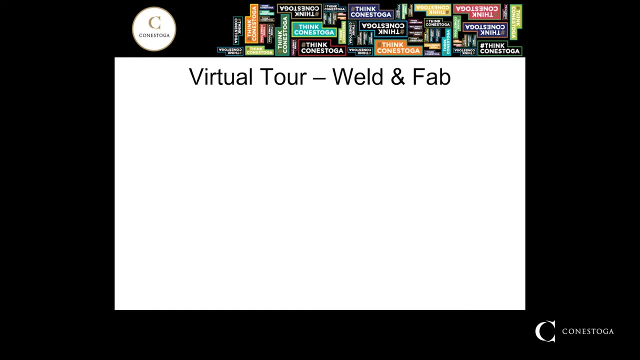 don't use these large rooms. The welding programs typically use a smaller classroom. We don't have that large number of students in one group. Now we're going to go into the welding and fabrication areas Again. in our program we're not just welding, but we also do metal fabrication. 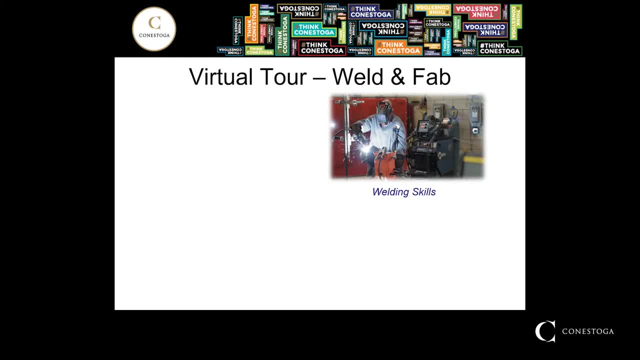 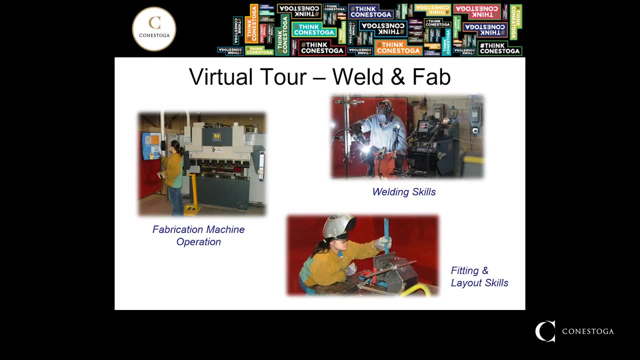 Obviously, welding skills are very important. It's a heavy emphasis on the first year, The first year of the program, But we also teach fabrication machine operations. This person is creating a metal part that's been formed on a press break. Once the pieces are created, they may have holes in it. 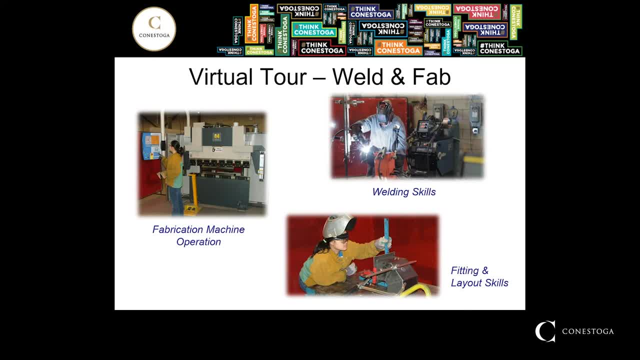 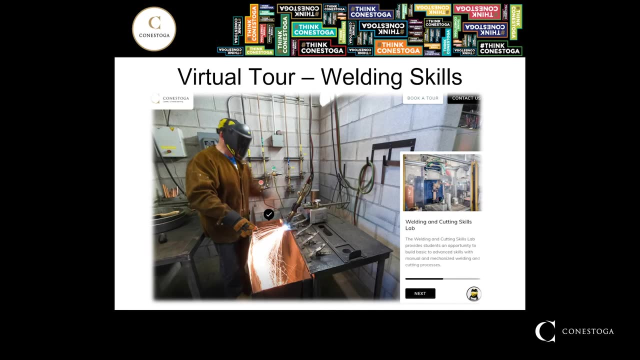 They may be bent, They may be rolled. All the pieces are assembled and tacked together. So fitting and layout skills are extremely important in our industry. Each of our students, Each of our students, Works in a welding booth. The welding booths have a number of different welding processes in them. 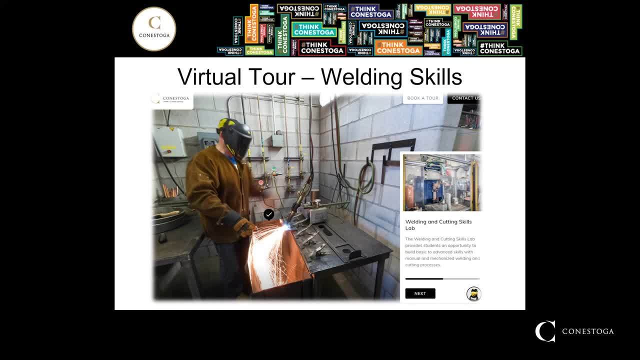 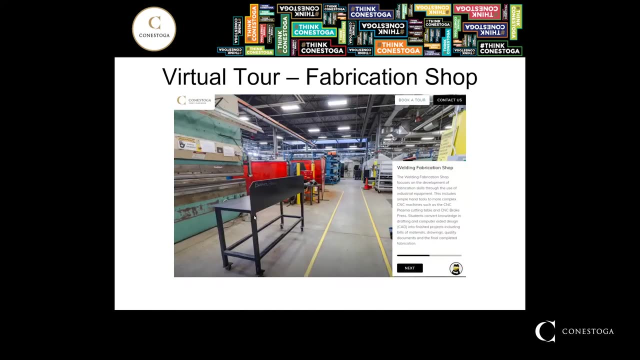 Maybe gas tungsten arc welding, shielded metal arc welding, gas metal arc welding, flux cord arc welding and thermal cutting. There are 45 booths similar to this out in the welding skills shop. Now I'd like to take you for a tour of the metal fabrication shop. 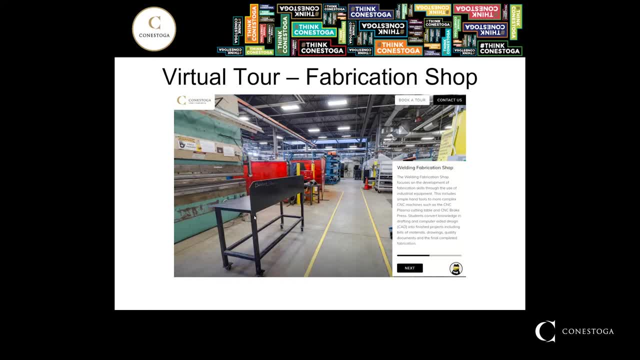 Go straight down that aisle way, You can see some welding booths. There are 45 welding booths in the welding skills shop. at the back, Closer to the camera, is our metal fabrication shop. To the left you can see a bunch of orange screens. 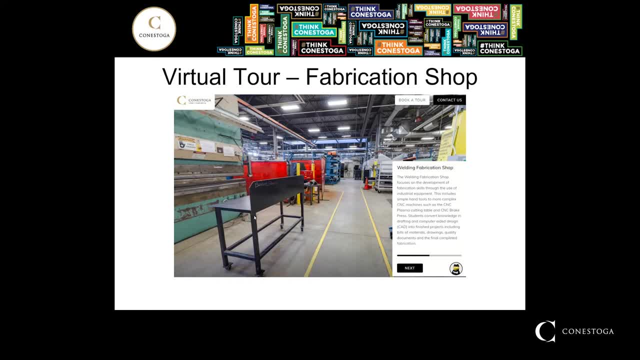 They're surrounding our plasma cutting machine. That's a CNC plasma cutting machine for cutting flat plate into shapes. As we look through the shop we can see the large machine there. That's a press break for bending metal. That can bend steel and metal. 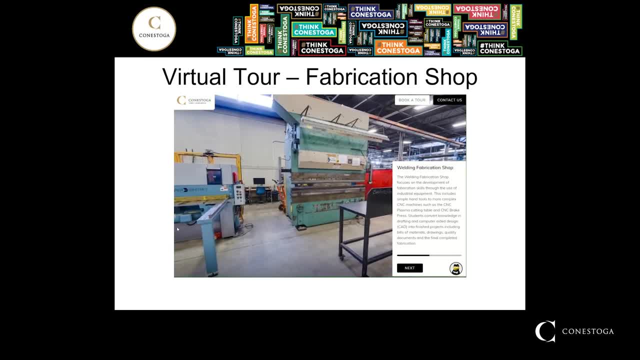 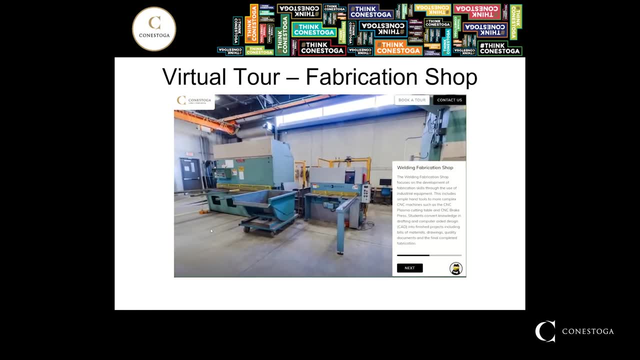 That's a press break for bending metal. That can bend steel and metal steel up to three-eighths of an inch thick. That's a sheet metal shear, the smaller machine And the big machine. there is a plate shear. That's for cutting steel three-eighths of. 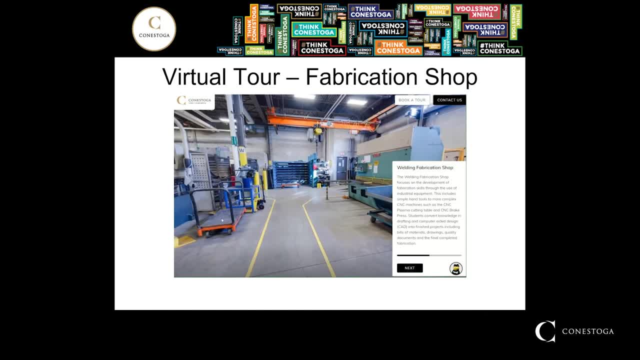 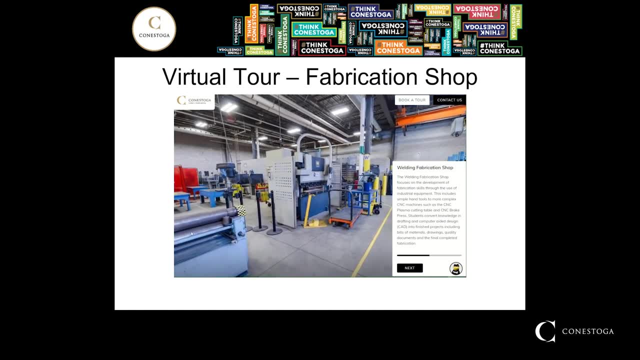 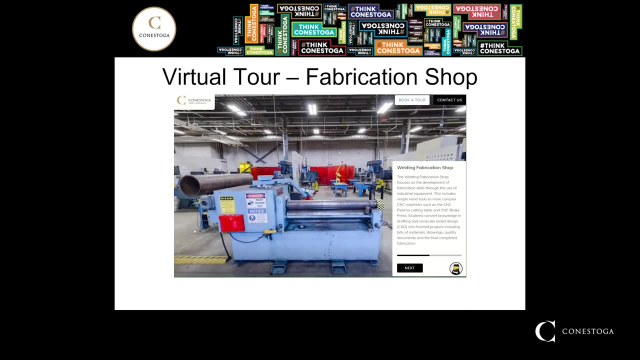 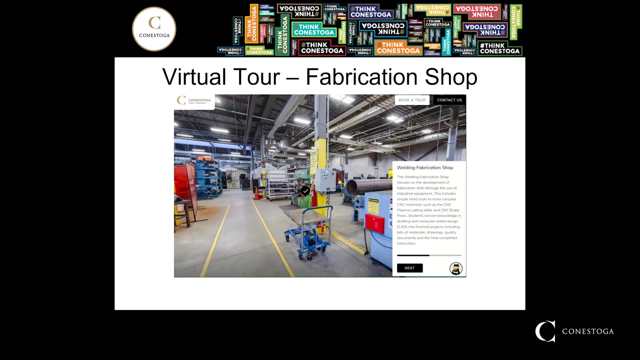 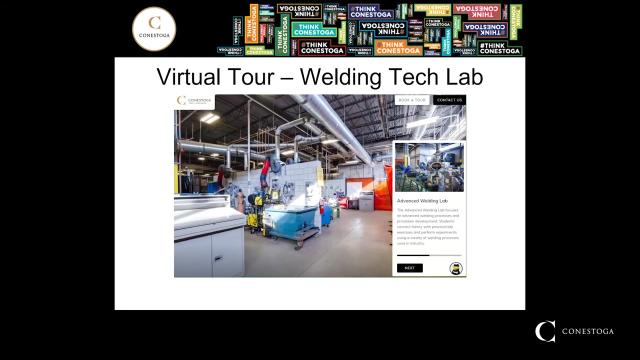 an inch thick. You can see the overhead crane and some material storage areas. That's a CNC press break for bending steel. There's a plate rolls and in behind it you can see some workstations for students who are doing their fitting projects. Next we'll have a look around our welding technology lab. This lab is unique in Ontario. 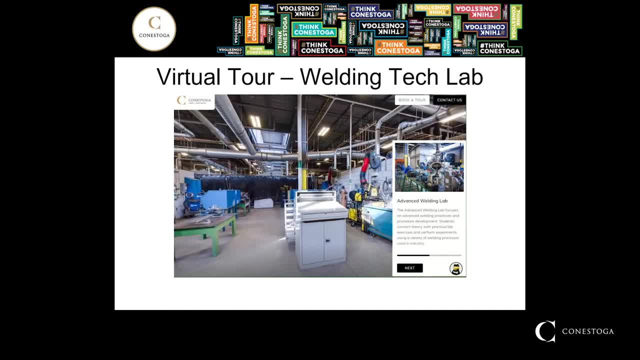 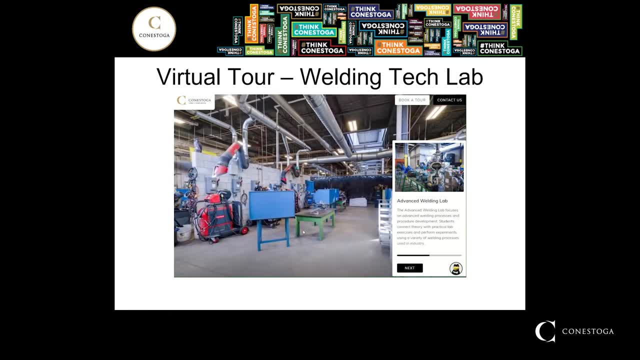 and probably in Canada. We have a variety of different advanced welding process capabilities in this, in this facility, You can see different brands of welding machines here. These are advanced machines, so these aren't your regular welding machine. They could do pulsing. they can do different welding processes that maybe you've never even heard. 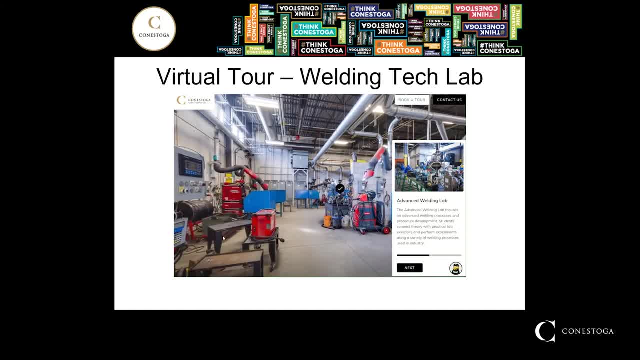 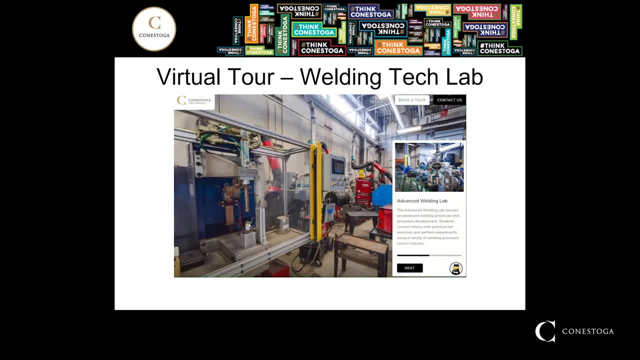 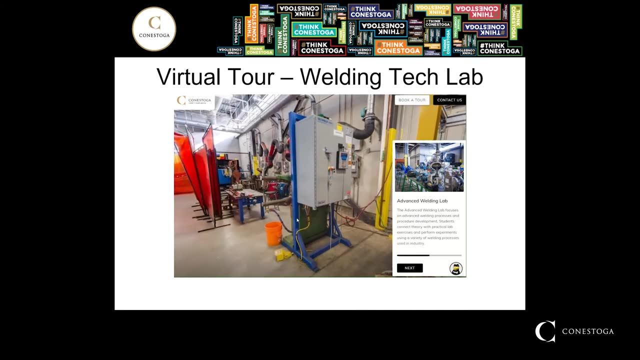 of. Over there you can see the ventilation systems and it's over top of some advanced controlled machines- The computer controlled machine. there is a spot welder, There's another spot welder And in behind you can see some other equipment. We have a variety of different. 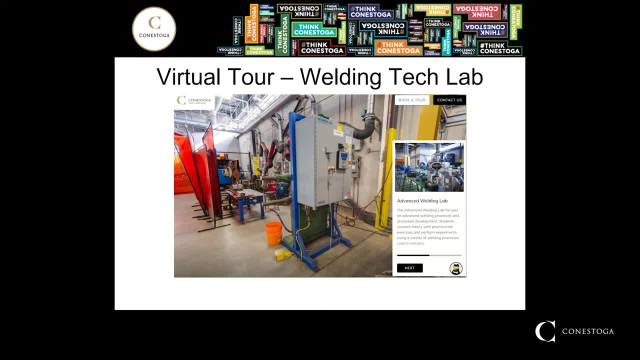 welding processes. We can weld plastics, we can weld heavy plate, we can weld stainless steels, we can weld aluminum, we can weld all kinds of metals. So again, it's a very unique facility. It's our welding tech lab. Conestoga College is also fortunate to have 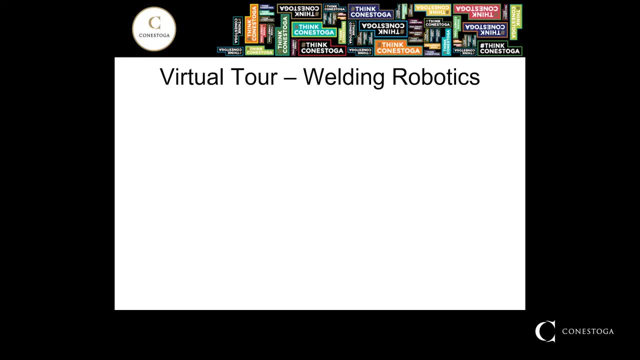 one of North America's top welding training facilities for robotic welding. Here we have students programming one of our welding machines. This is one of the most advanced welding machines in North America- One of our six arc welding robots. These students are programming using 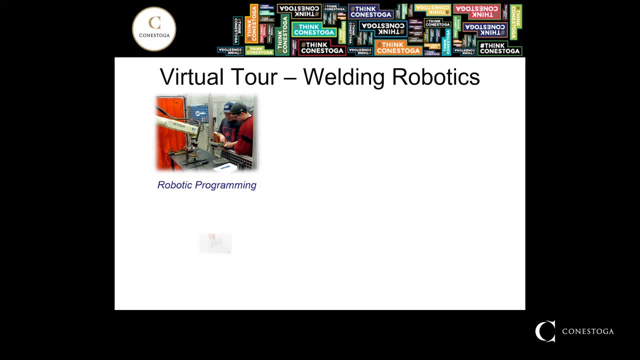 a teach pendant. We also teach students to program from 3D models. Here we generate a 3D model with software such as SolidWorks and introduce that part into a virtual reality world with a virtual reality robot. We have a real robot just like it, but in the virtual 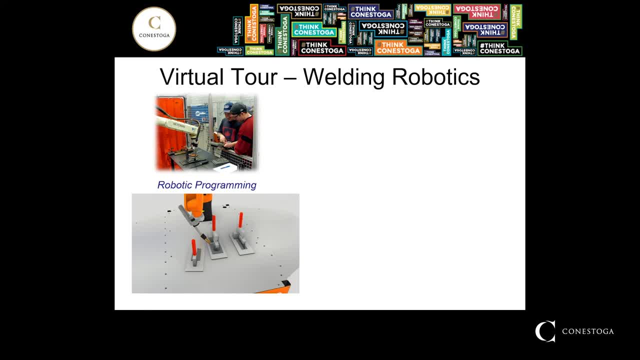 reality world. we can test the robot's program without ever actually having the real part in our hands. Once the students learn how to program that robot, then we can take that program and download it to a real robot. Here you can see the same part: a little pipe being welded, getting. 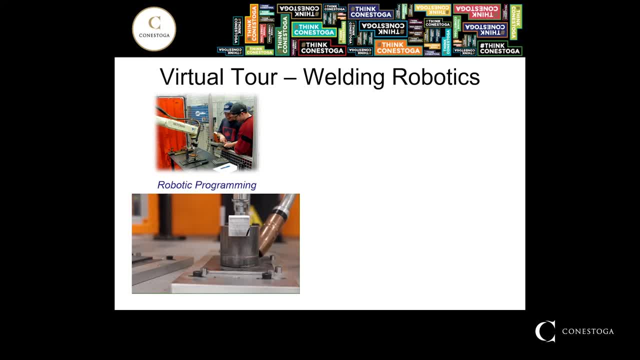 ready to weld by our arc welding robot. That program was learned in a virtual reality world. We've had lots of success with this, but this is a specialty of our students in our manufacturing engineering technology- welding- And once we are prepared to get involved in a robot, we 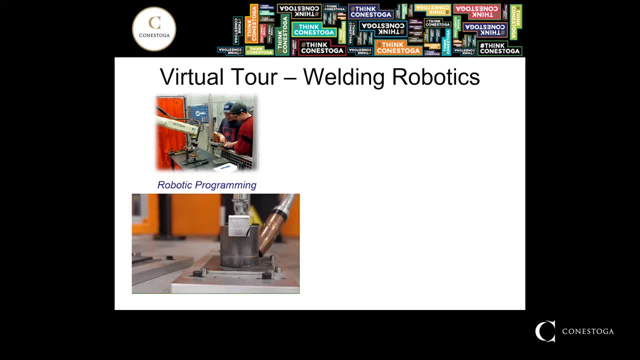 can also bond it together. This is what we call a robotic welding Once the students welding robotics program. that's one of our three-year engineering technology programs. we've also had success with additive manufacturing. here we're doing 3d printing of metals using an arc welding robot that the students have learned to program to do the job. 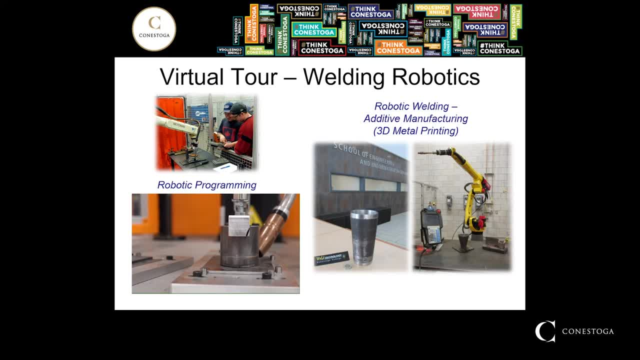 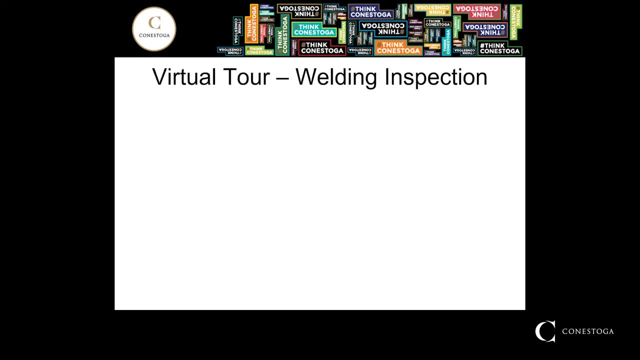 the mug you see was created out of stainless steel by our students using that welding robot. conestoga college also has a lab dedicated to welding inspection and metallurgy. we have a program, a three-year program, called welding engineering technology inspection. in that program students study, for example, the metallurgy of welds. here you can see a student. 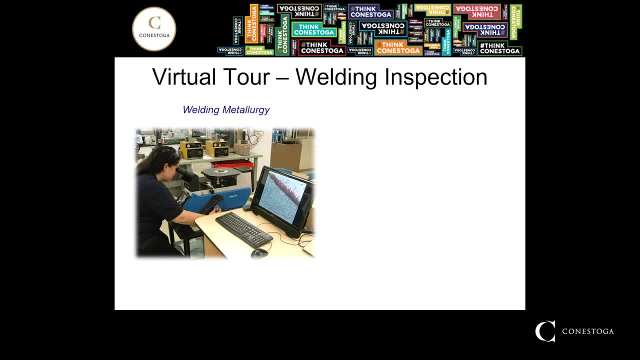 looking through a microscope at a polished sample of a weld to try to understand the metallurgical structure of the weld. the image has been projected up onto that computer screen. students in that program also study various aspects of welding inspection. here you can see a group of students studying the ultrasonic inspection of welds. 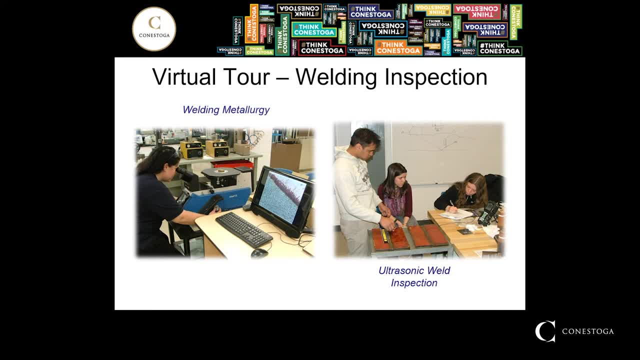 this method is similar to medical ultrasound: it sends sound waves into the steel and if there's any defects in the weld, they bounce back and send a signal to the electronic equipment. understanding these topics is a bit more technical than learning how to weld, so you have to think. 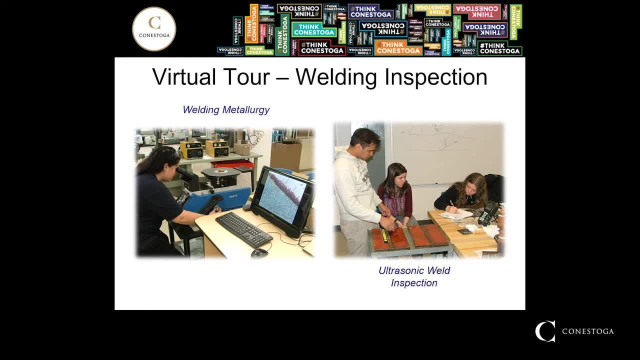 about this, but it is an option for students graduating from either the welding and fabrication technician or the welding techniques program if they want to progress to these programs in engineering technology- either an inspection or welding automation, welding robotics- that's an option that's still open to you. the career opportunities for welding techniques grads are: 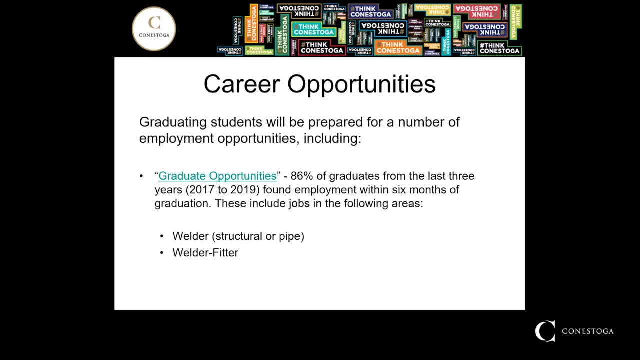 varied. most of them are looking for jobs in the welding industry. obviously, these jobs are generally called welder or welder fitter, although many companies have different names. in terms of our graduate success, 86 of graduates from the past three years found employment within six months of graduation. despite the covet epidemic, the job market 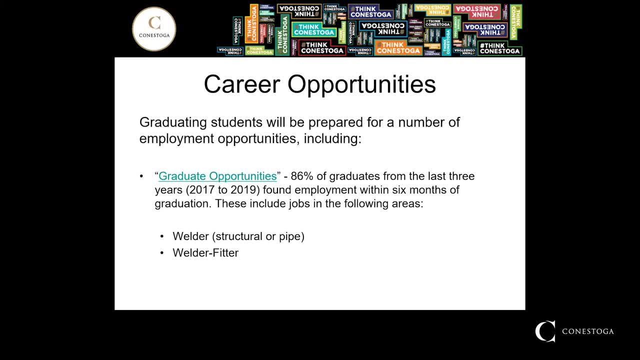 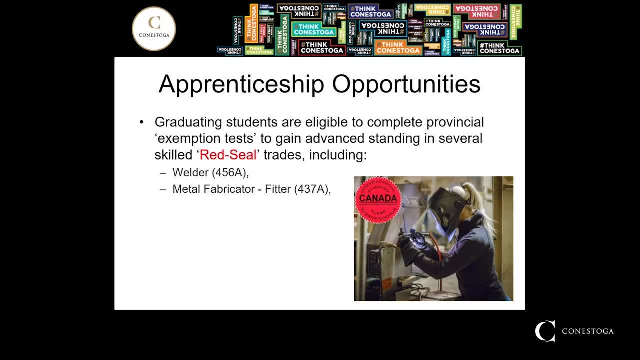 for welding and metal fabricating trades are still strong. in this area. a lot of students who are working in the welding industry are expected to be more successful than others in the field of weld engineering. in the field of welding and metal fabrication, there are a lot of students who are 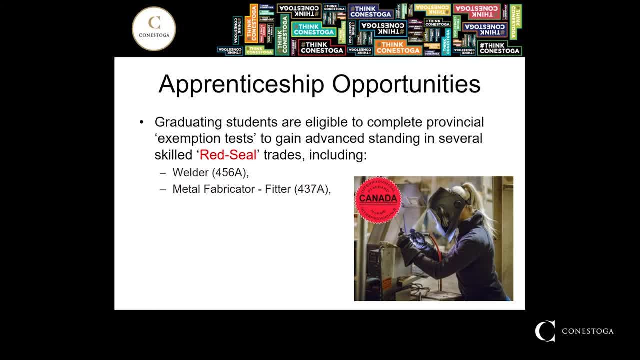 are entering the trades are always asking questions and interested in the opportunities to be a journey person. how do we become a journey person? well, that's through an apprenticeship in Ontario. there are two specific trades in the industrial world that are targeted at welding and metal fabrication. that's. 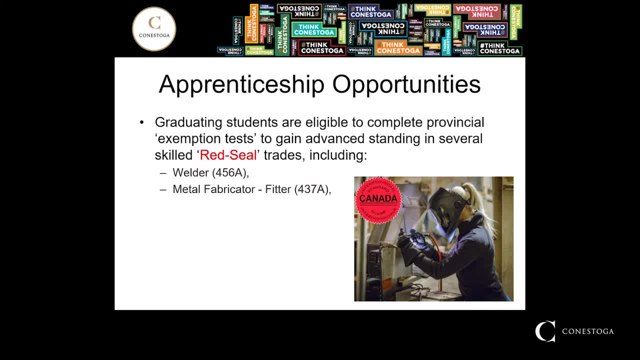 the welder and metal fabricator fitter. these trades are designed to bring a person up to a level- that's what we call at the Red Seal, or interprovincial level. that gives you the opportunity to work across the country applying the trade. in our programs we've designed the content to be compatible with the apprenticeship. 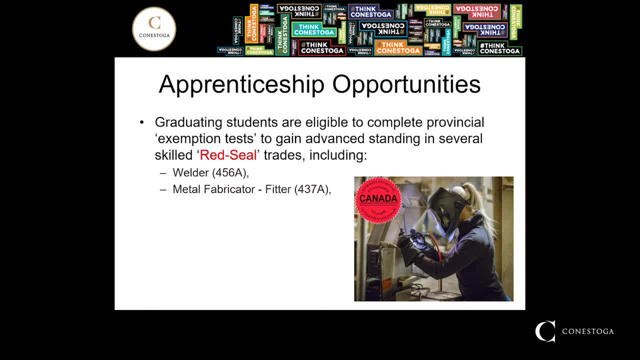 trades. this provides the opportunity for graduates to proceed over through an exemption exam to enter an occupational trade and find employment as an apprentice. by being an apprentice you can then complete the training and then complete the apprenticeship and then complete the trade by learning, learning the on the skills portion and at the end of that. 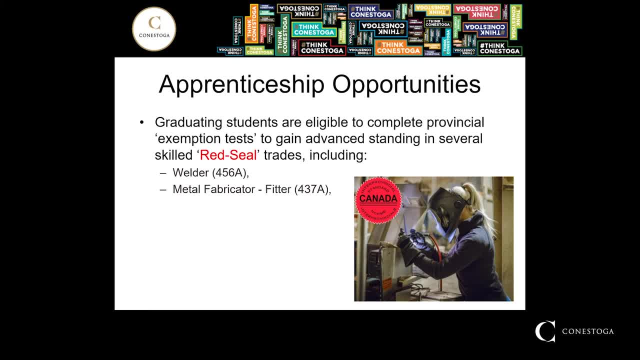 you can write an interprovincial exam again. the two primary trades that were focused on in our area and we deliver at Conestoga College are the welder and the metal fabricator. there are also many other related trades. I've listed some of them here: construction, boiler maker, iron worker, steam fitter and sheet metal. 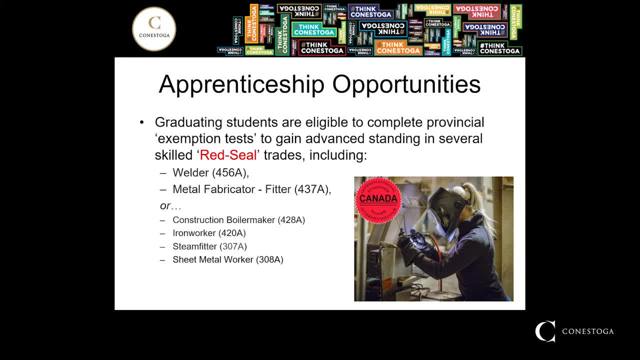 worker. there's other ones as well, such as a construction millwright. a lot of those trades do a significant amount of welding. a construction boiler maker. it doesn't say they're welders, but essentially they're metal fabricators and they have welders working alongside them. same for 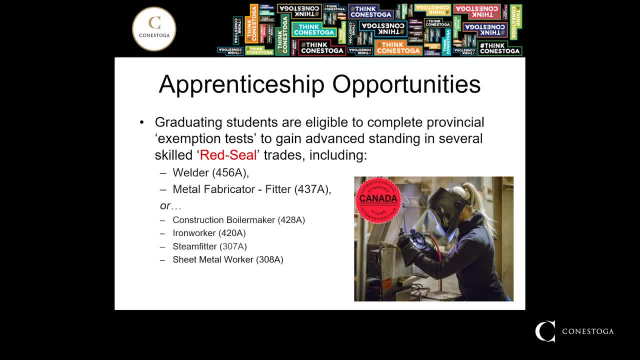 steam fitters, and that would be a construction trade where they fit pipes and weld them together. iron workers are for primarily working in the structural steel world, and sheet metal workers work on thin, thinner sheets and thinner gauges of metal. so these trades all do welding. they all have aspects of what we're. 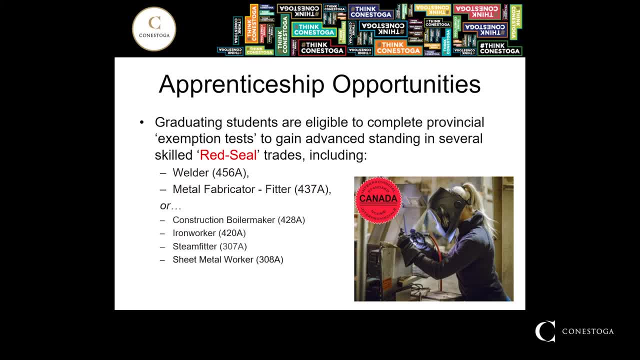 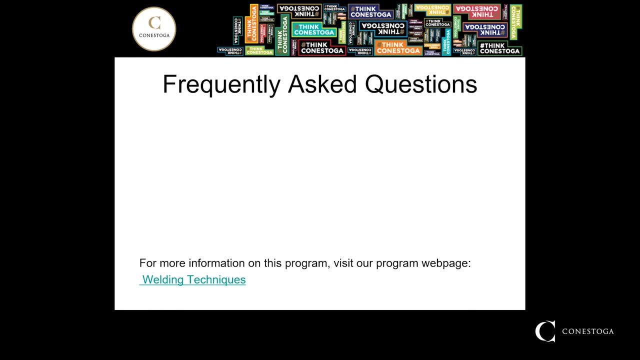 teaching and they're all related to welding and they're all related to the steel world and many of our graduates have gone on to those career paths as journey people in these red seal trades. just going to go through some of the frequently asked questions that people have and try to provide a quick answer, but again, more information can be found. 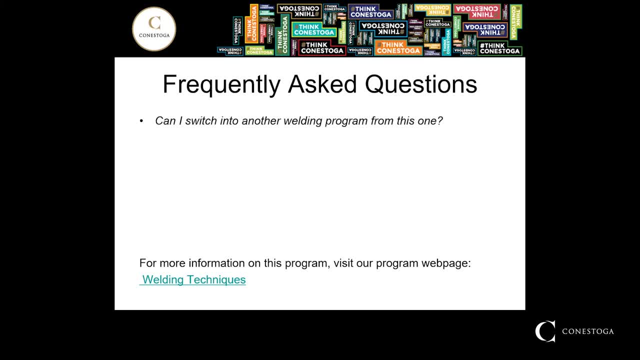 from the website. can I switch into another welding program from this one? and that's an emphatic: yes, the programs that we have at Conestoga College are integrated so that students who complete year one of any of the programs that were listed can then transfer their credits into the second year of another program. 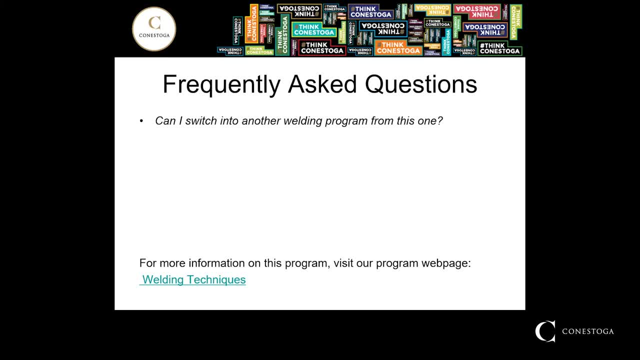 provided you have seventy percent in math, both math courses in year one. you can take your credential there in the mathematics and apply it to the engineering technology field if you choose, or you can take the two-year welding robotics program. how much welding will I learn? I'm going to learn all the basic welding processes: shielded metal, arc welding or stick welding, gas. 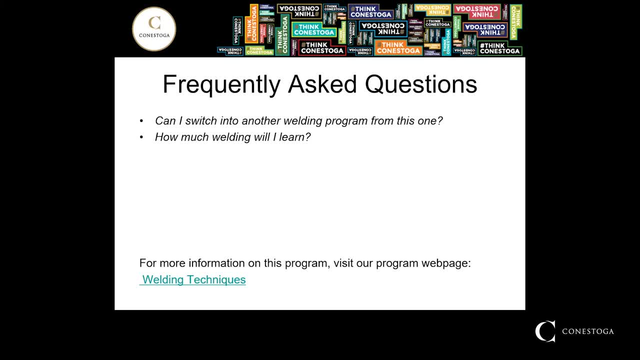 tungsten arc welding or TIG welding, MIG welding or gas metal arc welding is a proper name: flux cord arc welding. all of these are welding processes that we focus on in first year. we also focus on metal cutting techniques and everyone also takes a metal fabrication course, so there's a lot of 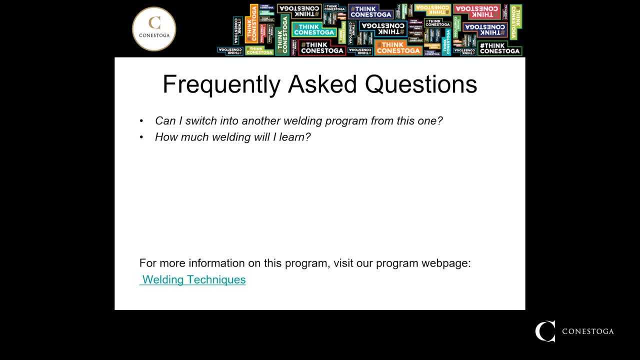 welding. over fifty percent of the first year of the program is in the welding skills shop. will I earn welding tickets? well, that's a trade qualification. there are various organizations that sponsor welding qualifications, and the primary one in our area that you'd be looking at would be the Canadian welding Bureau. we do offer Canadian welding Bureau testing. we can't. 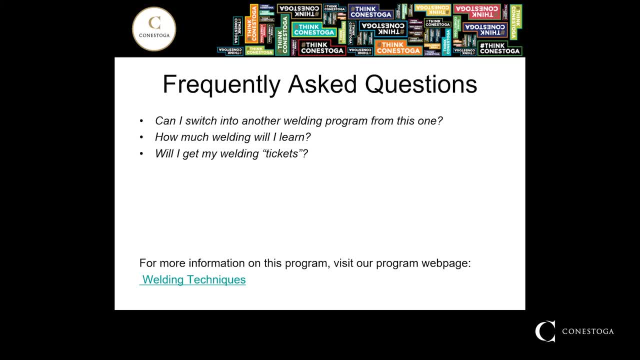 do the testing ourselves. the Canadian welding Bureau has to come in and actually do the testing, so it's an extra fee, but we do provide the opportunity for the Canadian welding Bureau to come in and test students near the end of the program. are there other credentials? once I'm finished, as I mentioned, the opportunity to to apply your trade. 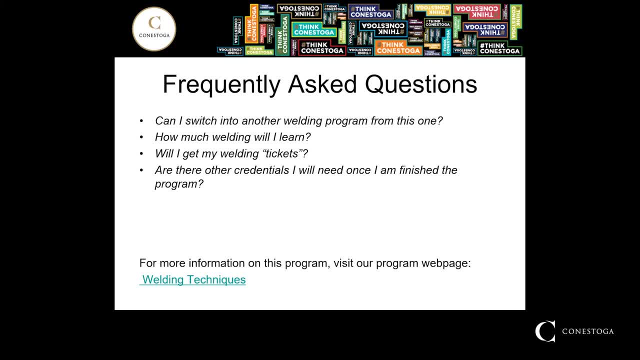 and and go for an apprenticeship and earn a red seal is one of the primary targets that a lot of graduates have. so yes, there are other credentials. you don't have to have them to get a job, but there are other opportunities and generally, obviously with more credentials or more skills, you have the 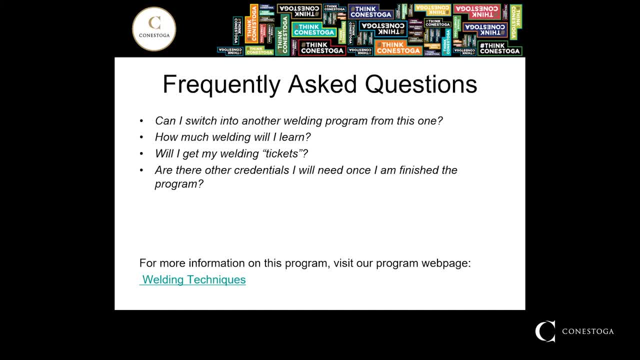 help you go on the pay scale that many companies are there apprenticeship opportunities. yes, many of our graduates, and again, we at Conestoga- we were one of the largest apprenticeship training schools in in the province and we do offer the welder and the metal fabricator fitter trade right in in the same campus and using the same 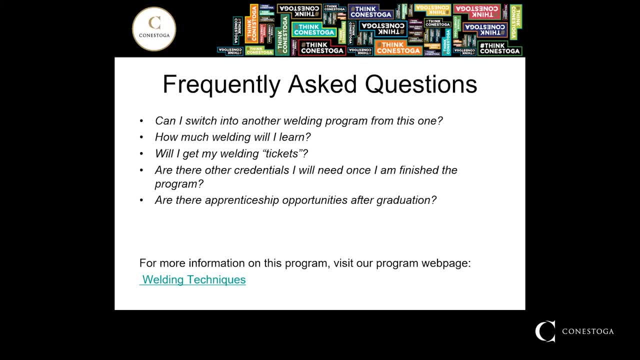 facilities that the students in your program would be using. we're also learning from many of the same documents and and learning packages, so we teach both. I teach in the apprenticeship program, I also teach in the post-secondary program, like your program, and so certainly the the opportunity is there to to move into apprenticeship. how much will I earn when I graduate? and that really depends on the employer. I've seen anywhere from you know low. on the low side you know sixteen, seventeen dollars an hour, up to thirty dollars an hour for new graduates. it really depends on the company and the type of welding you're doing. the higher 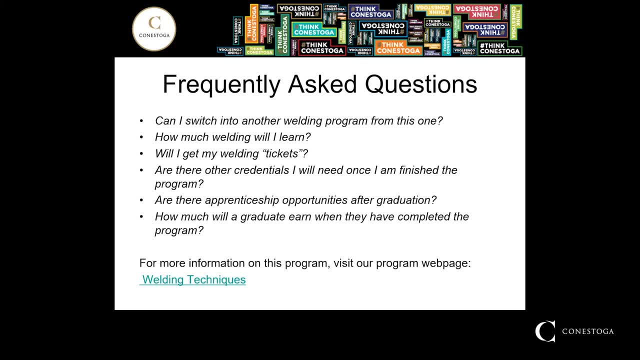 skills you have, the more credentials you'll have, the typically the higher you'll be paid. also, the the more critical that the product that's being manufactured. for example, you might be making a boiler for a for a nuclear power plant. well, that's going to have a lot higher quality requirements and 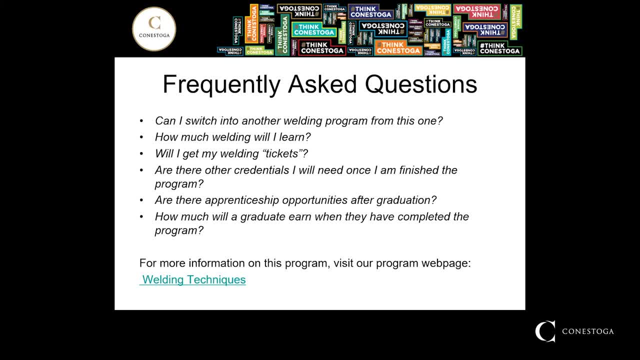 generally, the pay is going to go higher, but the expectation of the employer is also higher for welding and welding equipment. skill level, attention to detail, quality performance- all that stuff you're paid for the ability to do that. the opportunities are wide open, though. we've seen graduates who have earned very, very great wages not too soon out of school. 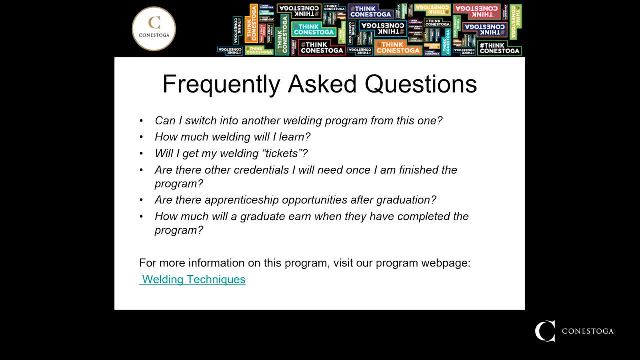 it really depends on the person and the opportunities and how they how they approach those opportunities. so there are some frequently asked questions and I hope I can respond to some of those here and I have been responding to them through this presentation. can I switch to another welding program after this one? 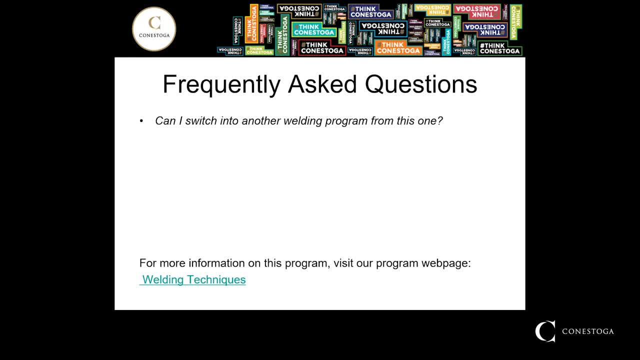 the answer is yes. we encourage that. we've had many students who enter the program to take a one-year welding certificate and then they apply those credits for advanced standing and other programs. this happens all the time within the this family of welding programs at Conestoga College. how much? 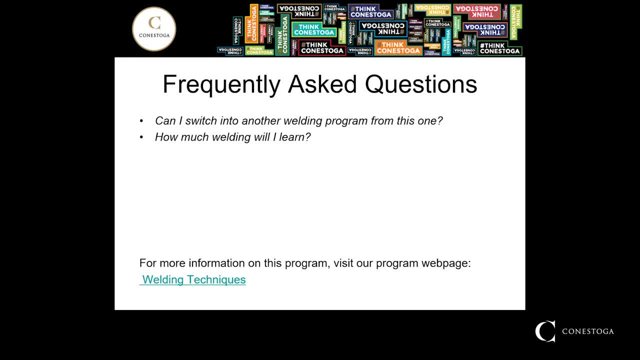 welding will you learn? you're gonna be learning all the basic welding processes, especially in first year. there's a heavy emphasis on welding skills and metal fabrication and cutting, so those thermal cutting processes are held in a different course, but the welding skills are taught, such as GMAW. 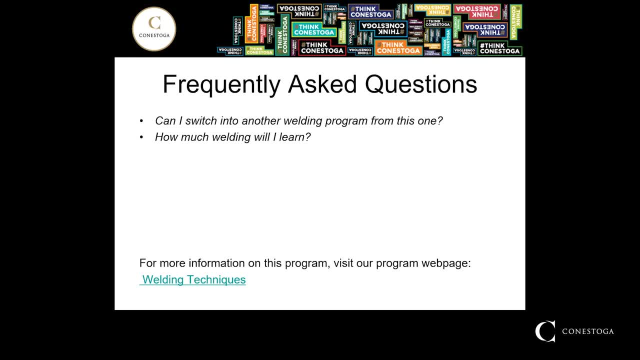 or MIG welding, flux-cored arc welding, gas tungsten arc welding or TIG welding, and shield of metal arc welding or stick welding- all the basic common welding courses that are that are taught in the first year of your degree. so that's a lot of information that we're going to be talking about in the next few weeks. 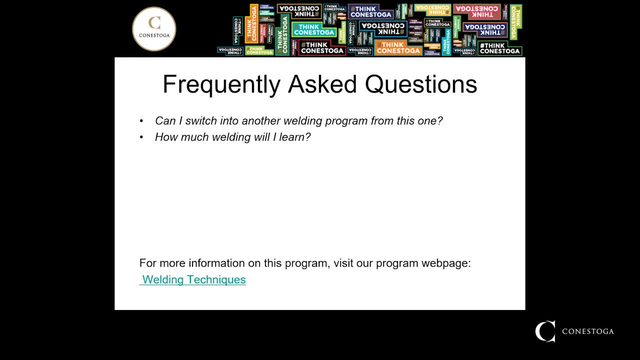 year of the program. over 50% of the first year is in the welding shops. will you earn welding tickets? we are CWB, Canadian Welding Bureau test center. so, yes, we do offer the opportunity for students to complete the, the practical tests that are required by the Canadian Welding Bureau to earn those. 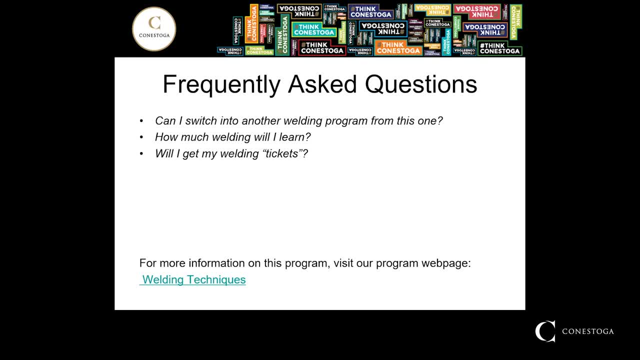 tickets. the Canadian Welding Bureau does have to, does have to manage those. they actually use our shop. they come in and we offer the opportunity for students to challenge those tests. no guarantee that you'll pass and it's up to the Canadian Welding Bureau who looks after the fees and whatnot. but we do. 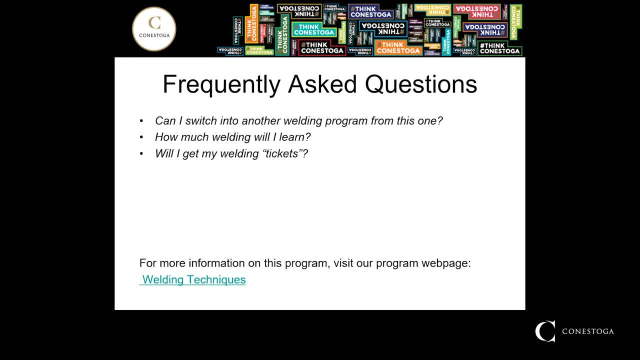 offer that opportunity. we are a CWB test center. are there other credentials that I need? not necessarily many students who graduate from our programs, they just go off and get a job. other students, as I'll mention in a minute, do decide that they'd like to become an apprentice and a journey person, and so that pathway is. 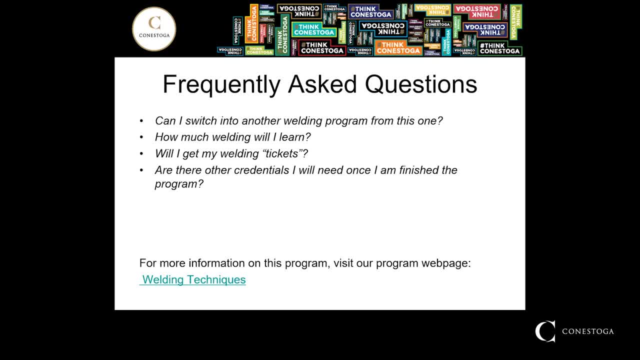 is also there. So, beyond the credentials of welding qualifications or tickets, there may be some need in some industries for other qualifications such as inspection or some kind of trade qualification, But generally it's not required in the welding industry, As I mentioned in previous slides.